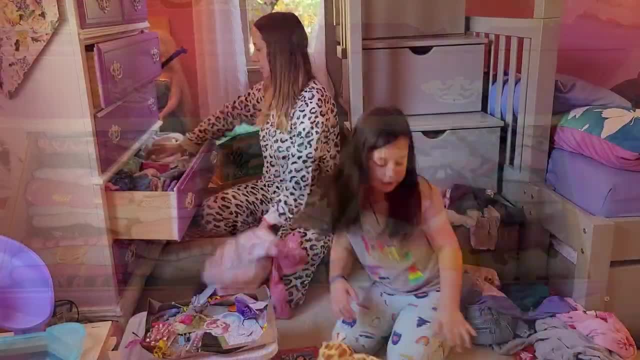 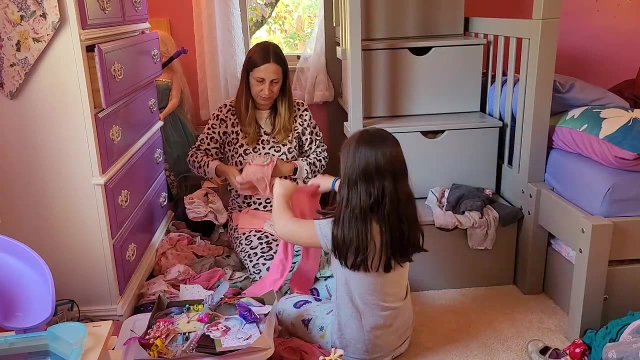 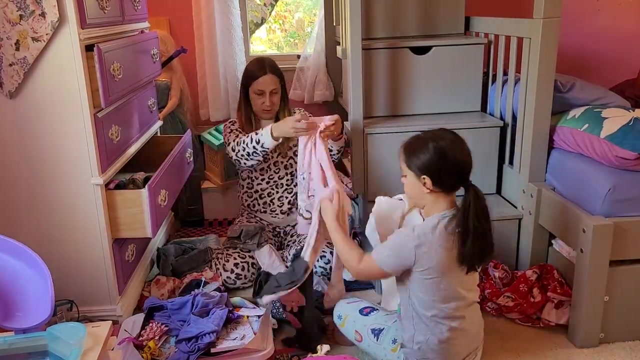 some drawer dividers that I got on Amazon. that made everything look even more neat and tidy. Then, with my younger daughter, we did the same thing, except we kept the outfits together, because toddler clothes tend to come with tops and pants, So we bundled those all together in little outfits. 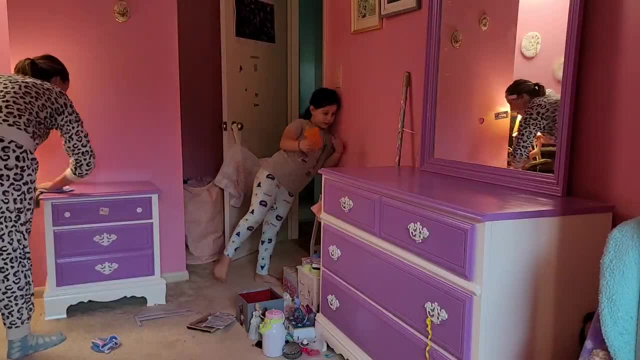 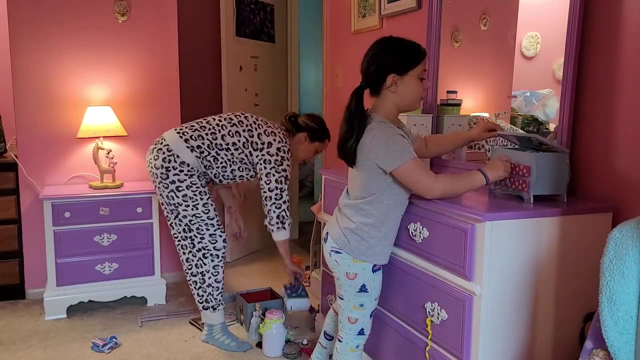 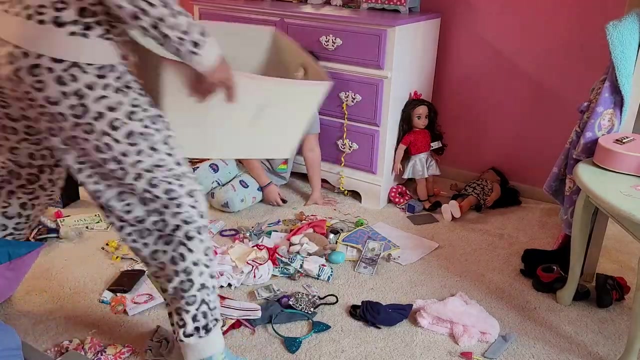 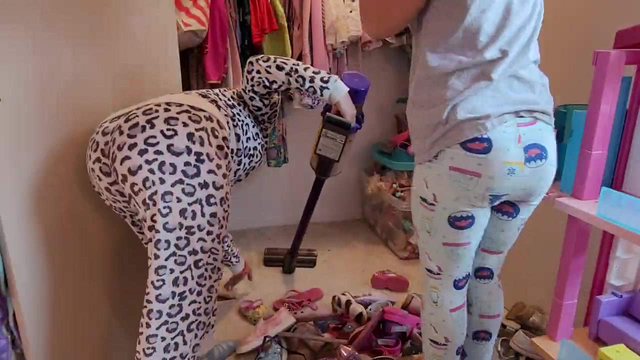 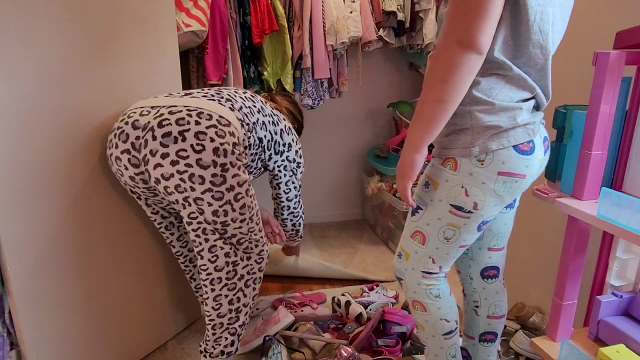 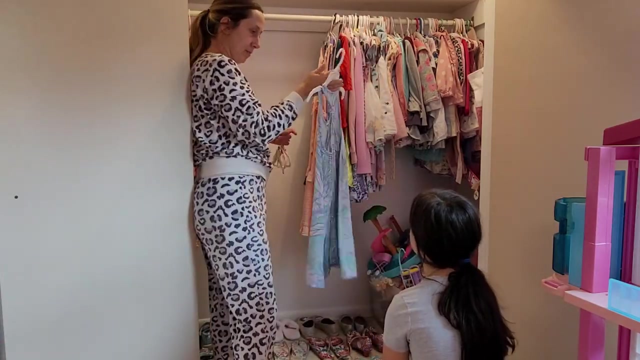 My daughter has a lot of toys and I brought in a smaller toy bin so she can keep her nicer dolls and their accessories separate. And a big surprise in the closet. I had no idea there were hardwood floors underneath these carpets. Next we went through the closet, got rid of everything that didn't fit anymore or had stains on it. 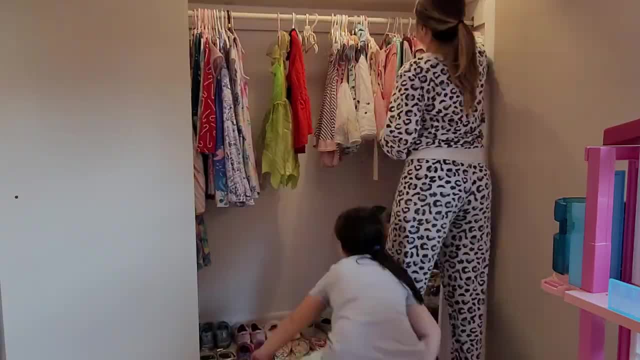 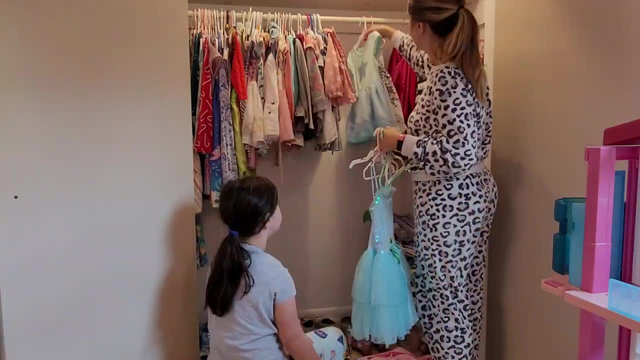 And I tried to take all the longer dresses and put them to the back, just so everything looked more neat and tidy. On the right side is my younger daughter's clothes. We just took out everything that doesn't fit her anymore and just tried to keep the short sleeve dresses separate. 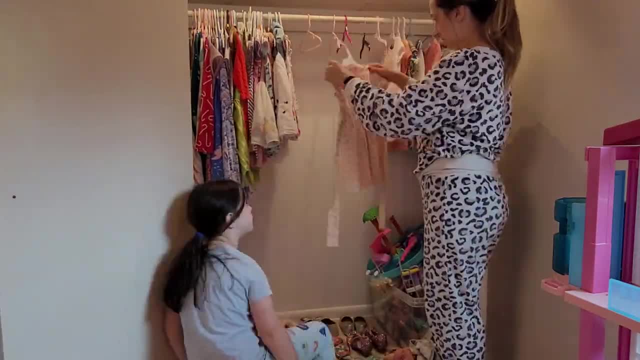 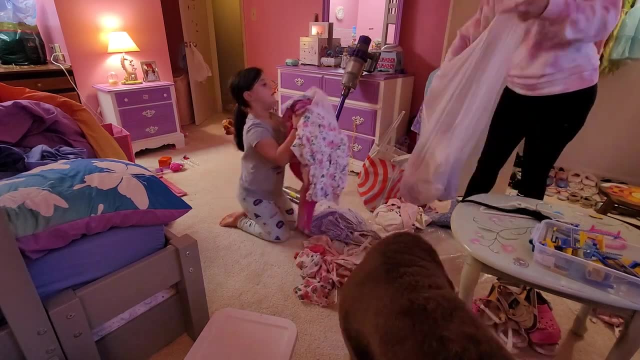 from the long sleeve dresses And I also took out all of the hangers that were either too small or just weren't needed, You know, the ones that kind of come with the clothes anyway. And then we bagged everything up and we will go through it to see what we can donate or give away. 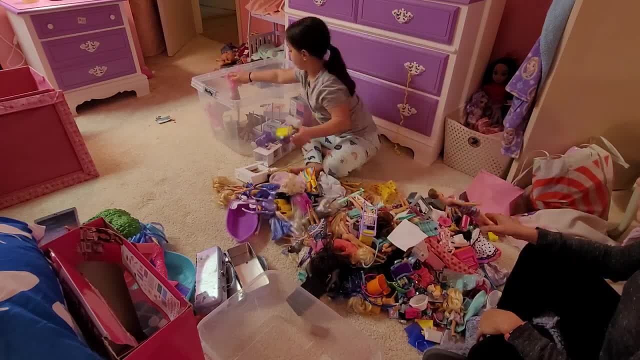 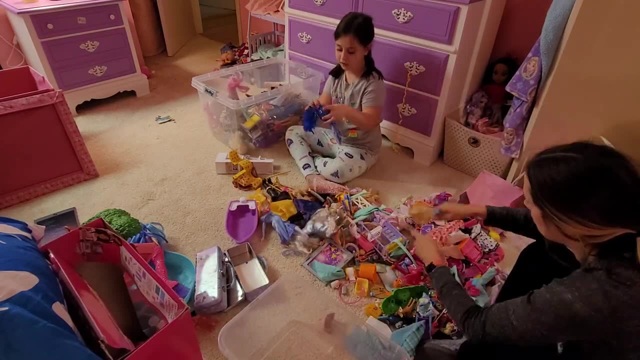 My daughters have a ton of Barbie stuff, So we separated all the bigger items into a large bin and then the medium size items into a medium bin And then really neat items. We got these pencil cases and put all the tiny little Barbie items into the pencil cases. 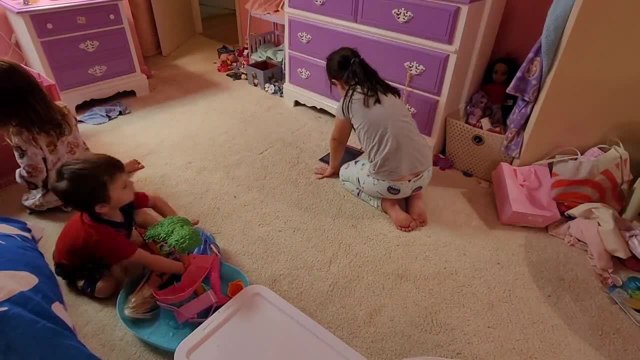 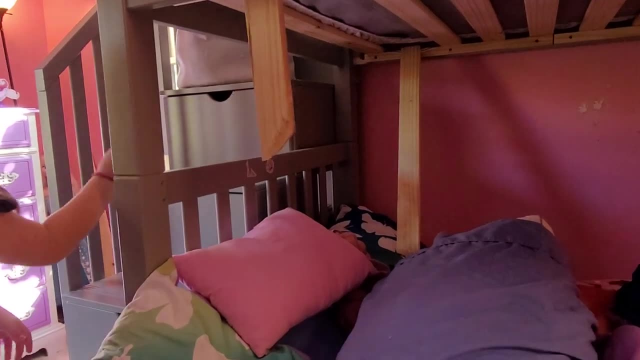 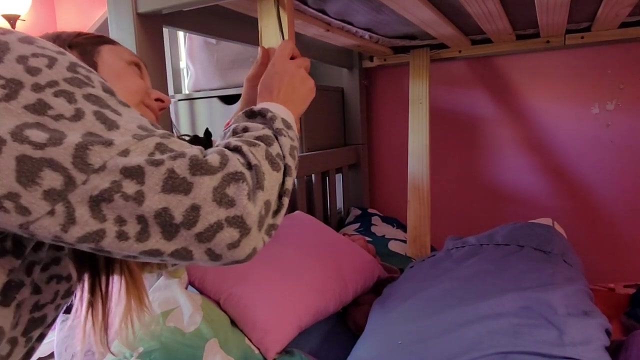 This way my daughter doesn't have to dig through that one big bin to find all the little tiny items And then making the top bunk bed. I actually snapped this piece of wood here by leaning on it. I think that it had a defect anyway and they are coming out next week to take a look and 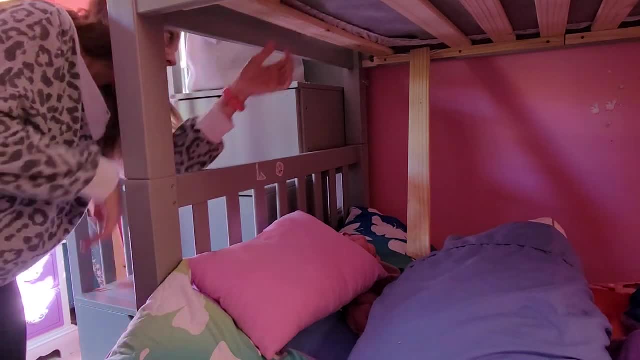 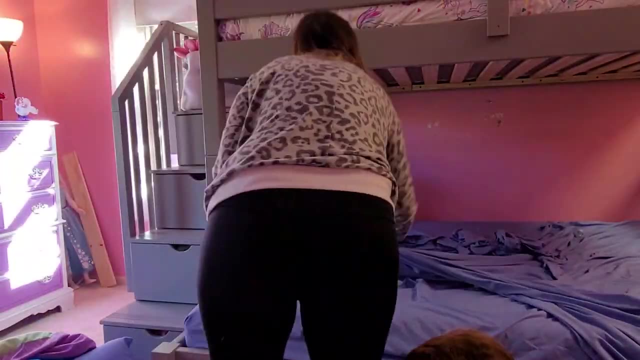 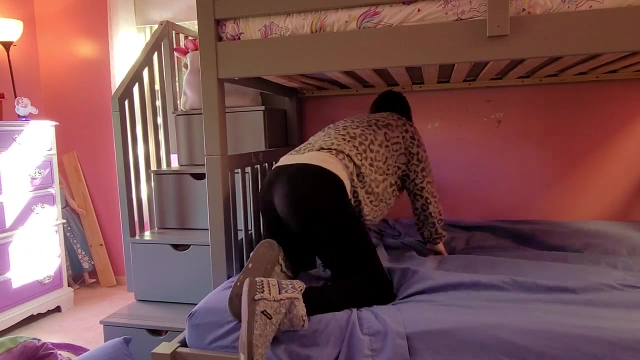 hopefully replace this, But I just tucked it up under here for now because I don't want to lose it, because I didn't know what else to do with it. Making a bed when it's against the wall is really tricky And that's how I ended up breaking that top piece, because you have to climb on the bed. 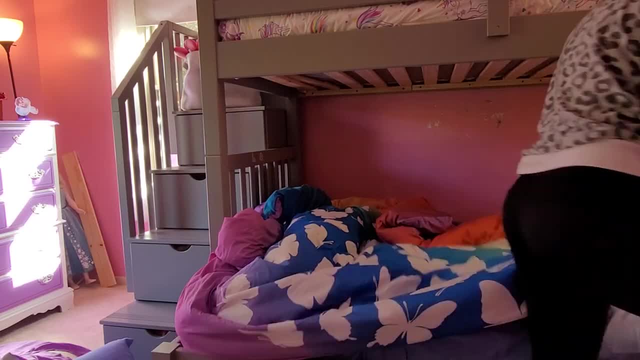 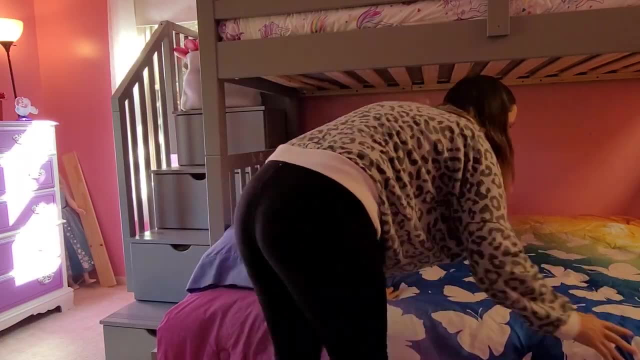 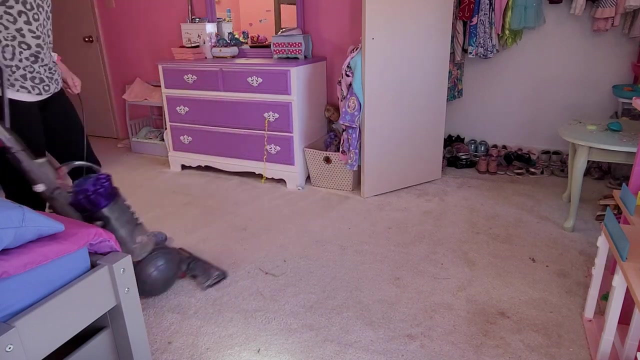 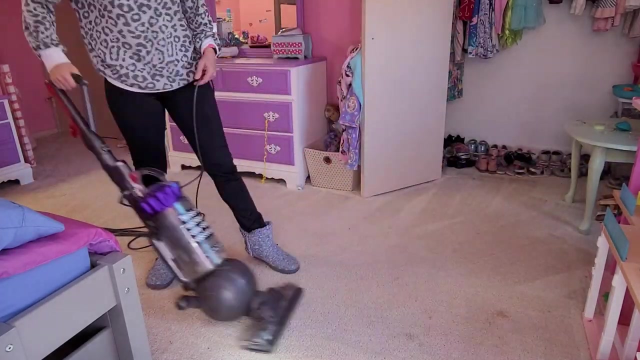 in order to reach the part by the wall. There are three more things I wanted to make for the ngoblas logo walk-on shelf tucked under the table, which means they had gotten to where I needed them. I'm sure they'll come back. 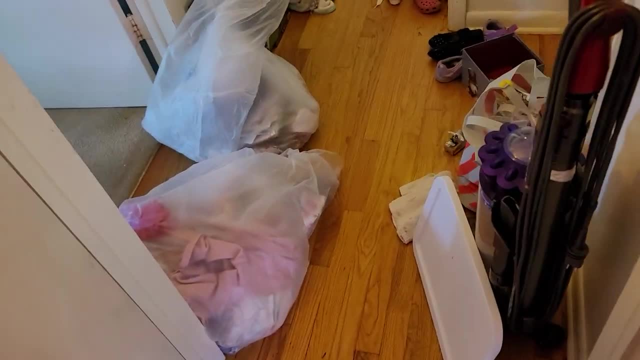 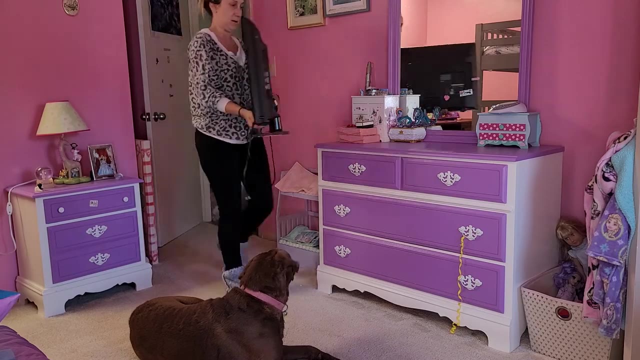 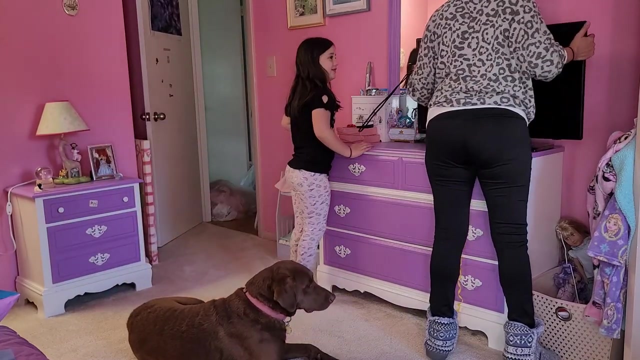 I also think that the intimacy was always so important to me. This is everything that we took out, or most of everything. I think I had already started putting stuff away. And the big moment: the TV. My daughter was so excited to finally have a TV in her room. 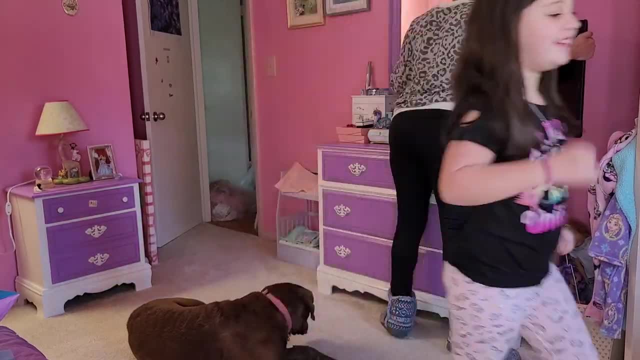 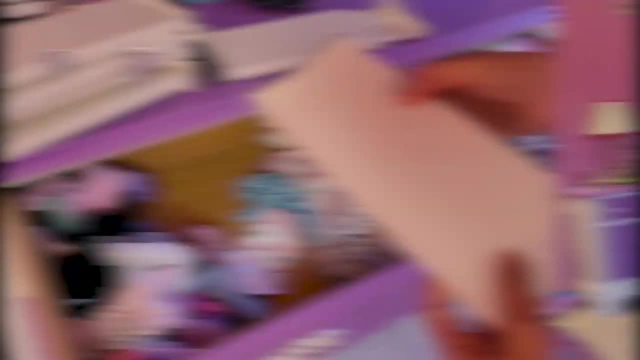 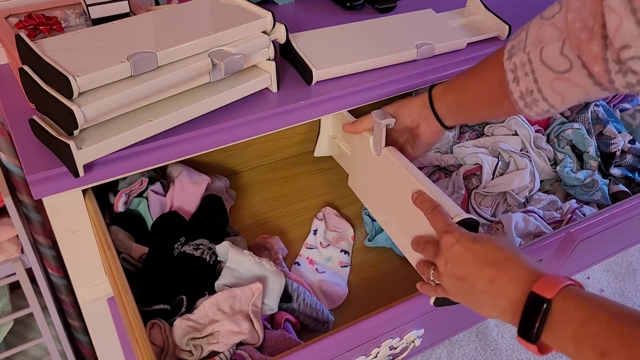 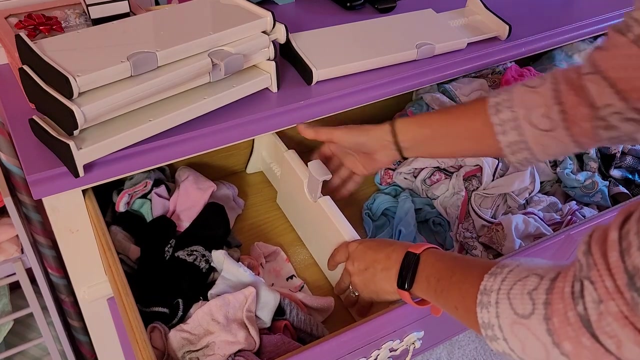 these are the drawer dividers i was saying earlier in the video. i got these from amazon and they are amazing. i wish i had them sooner. i don't know how i lived without them. so basically, you can just divide up any drawer into separate sections. it's so simple. i got these in a pack of 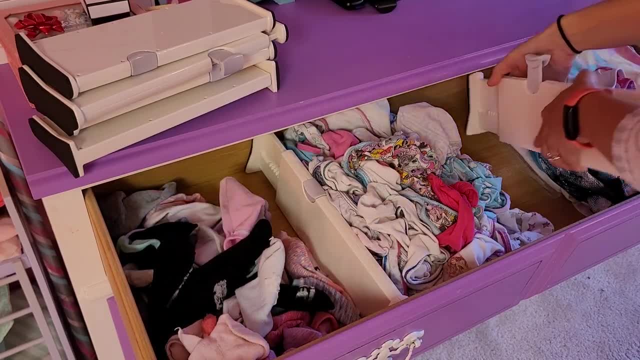 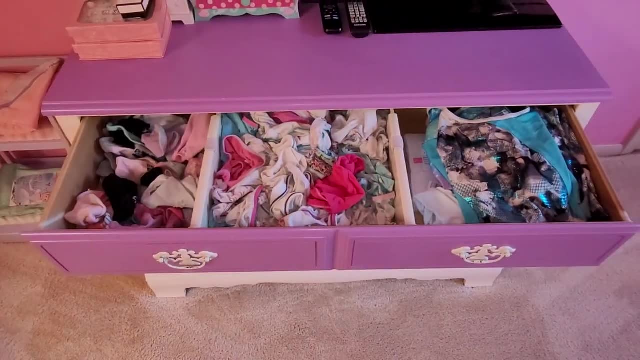 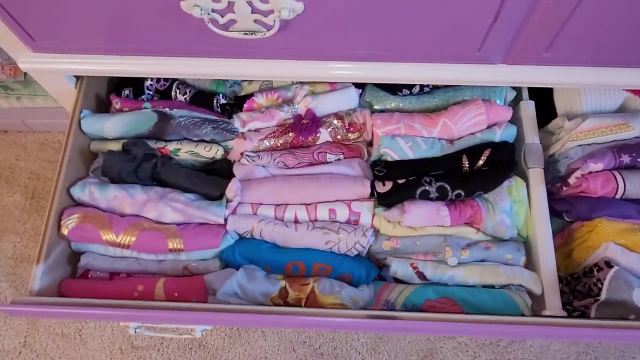 six and i do have the link in the video description. so i just put the underwear, the socks, her like bathing suits and leotards all separate, and then i also put one down here to keep her short sleeve shirts separate from the long sleeve shirts and i put a couple more of 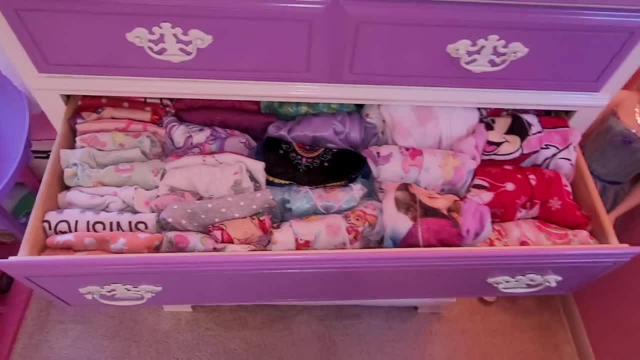 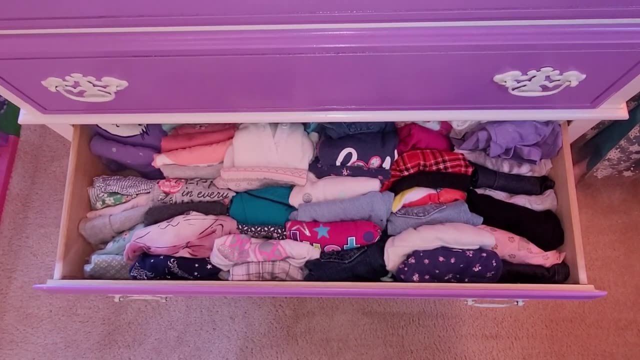 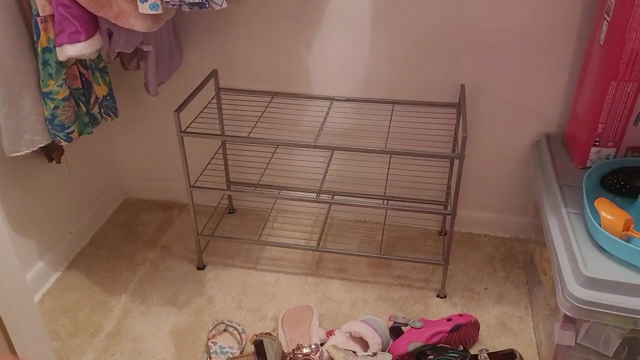 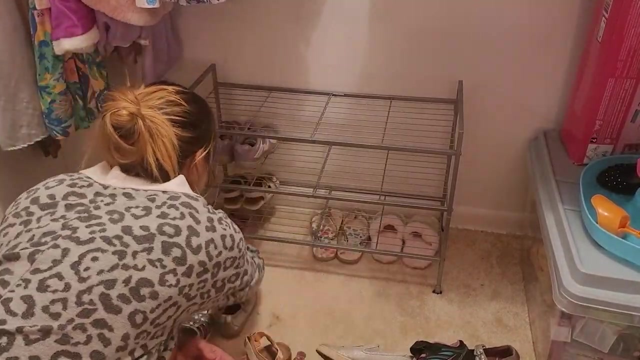 these into my younger daughter's dresser as well. and here are her pajamas, all nicely bundled up for her outfits, all bundled, and earlier in the video we had gone through the shoes, but they just didn't fit neatly in the closet. so i got this shoe rack on amazon. it was around twenty dollars. it took me about. 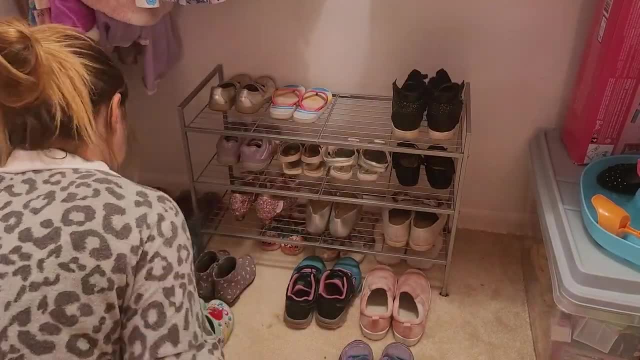 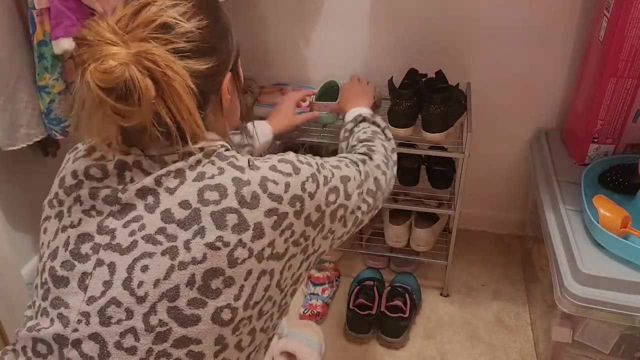 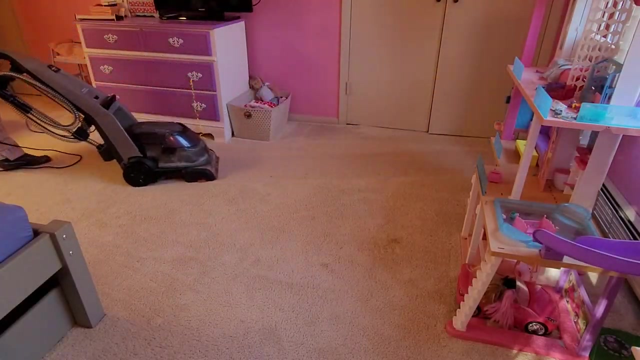 five minutes to put together and it's just great for little kids shoes. it really saved a lot of space in this closet and made everything look so much neater and tidier. didn't think the floors were that dirty, but there were a couple of stains i was trying to get out.